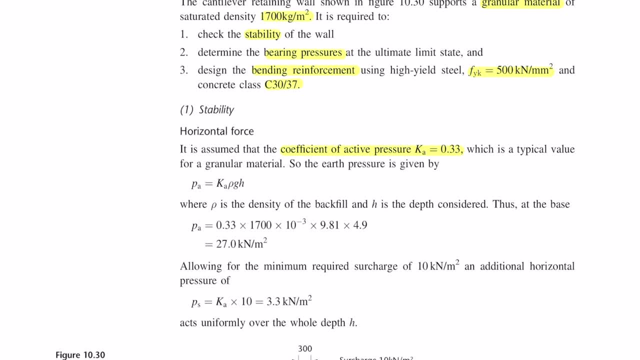 called active and passive pressure and because we're adding granular fill, we need to know what the active pressure of this granular fill is, and that's denoted by the coefficient Ka. In the middle we have a differential pressure difference. In the middle we have a pressure. 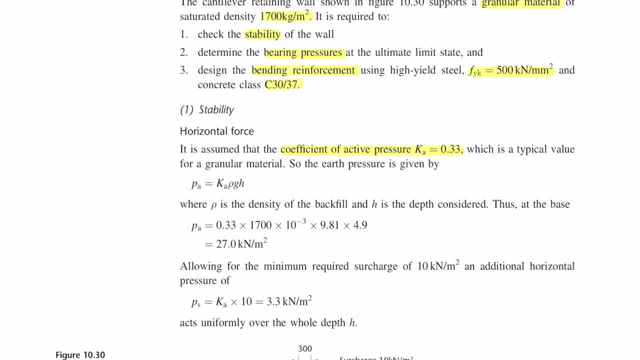 this instance, because it's granular fill, it's going to be 0.33.. There are two horizontal forces acting on our wall: one from the earth pressure or the soil and a second from a surcharge. The surcharge is essentially just the live load and if you imagine someone walking behind the retaining, 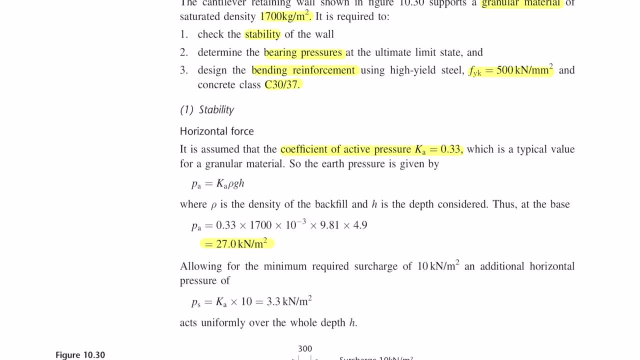 wall, that person is surcharging the retaining wall. So to work out the pressure behind the wall due to the soil, we use the equation ka, rho, gh. Ka is the active pressure, rho is the density of the granular soil, g is gravity and h is the height. Plug the numbers into the equation and 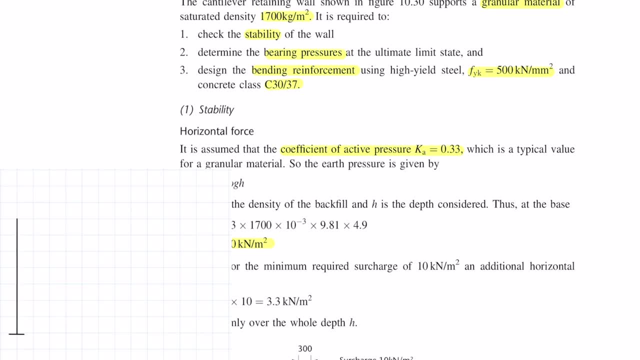 you get 27 kilonewtons per meter squared. Lateral earth pressure is distributed onto the wall as a triangle. Next we need to calculate the lateral force due to the surcharge, which in this case is 10 kilonewtons per meter squared, and all you do is multiply 10 by the 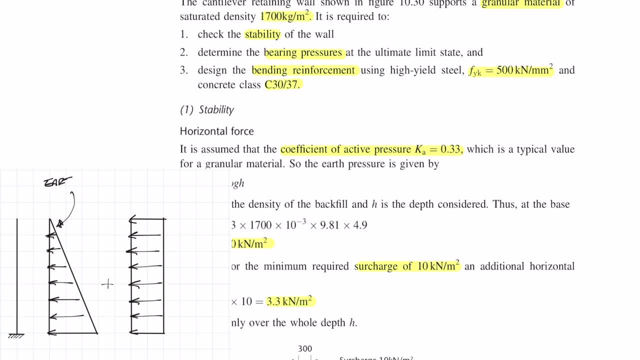 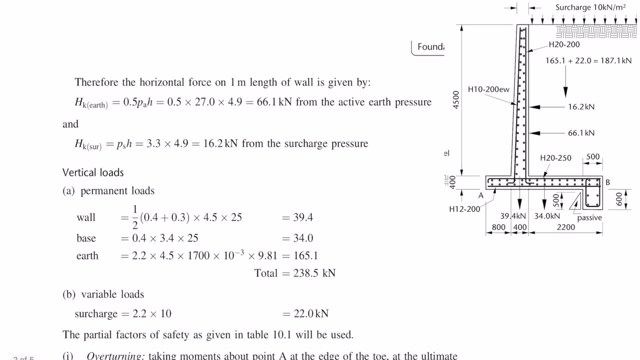 coefficient of active pressure to get 3.3 kilonewtons per meter squared, and this acts uniformly over the wall, so essentially it's a rectangle. So now we can actually work out the horizontal force from the pressures we had just calculated, and this is over a one meter length. 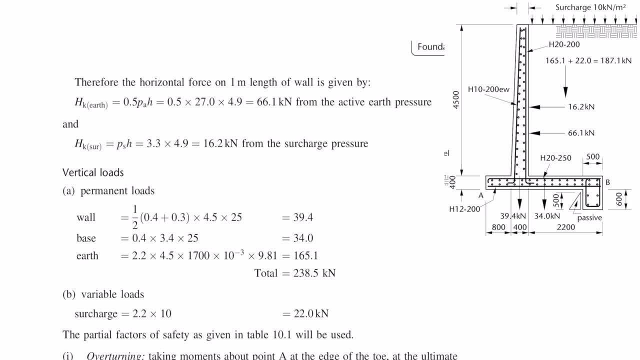 of wall. so essentially all we're trying to do is work out the force which is the area of the triangle or area of the rectangle. So for the earth pressure it's half base times height, so it's half times the pressure times the height, and the force due to the surcharge is 0.3 kilonewtons per meter. 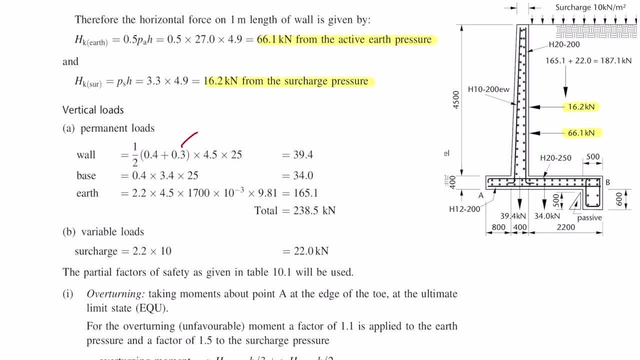 squared, which is just base times height. Okay, so now we can work out some of the vertical loads, and that's just going to be the self-weight of the retaining wall. so you've got to work out the wall, the base, and then you've got the soil pressure. that's obviously got a vertical element to it. 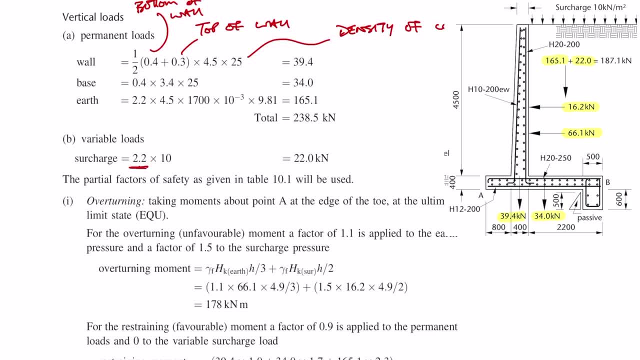 and then also the surcharge. Okay, so the first stability check is the overturning check. Now we're going to be taking moments about the point a, at the edge of the toe, which, if you didn't know, was the front of the retaining wall, and the heel is at the rear of the retaining wall. So when 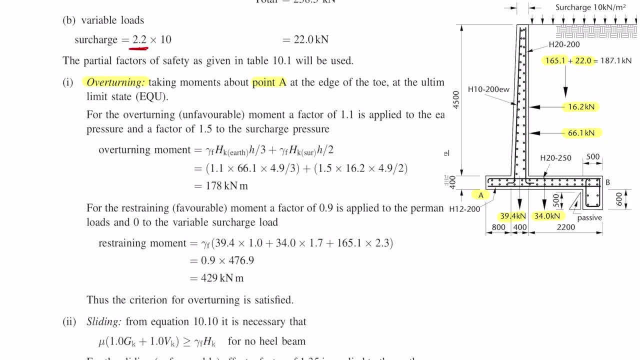 we start with overturning moments. you want to multiply up the unfavorable forces and the dead load factor is 1.1 and the live load factor is 1.5.. Now, with the restraining or the restoring moment, which is actually a favorable force, we want to apply a reduction factor of 0.9.. 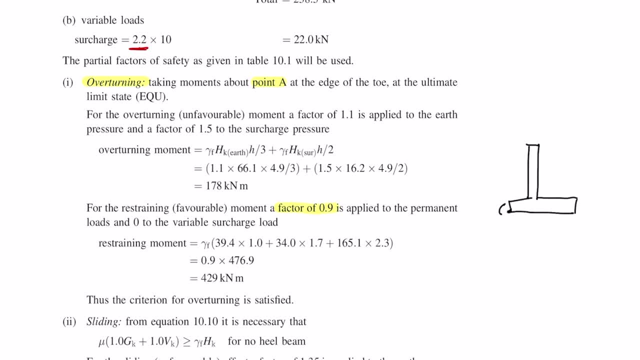 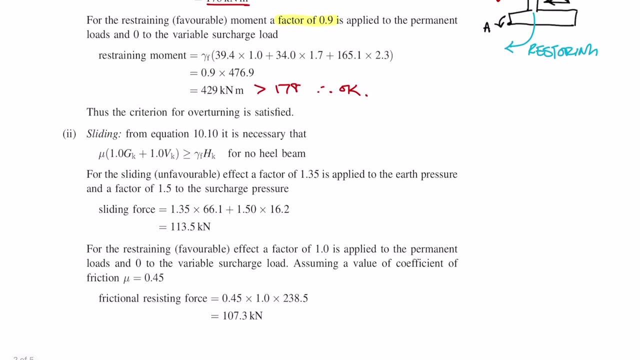 Now we only do this with the dead load and we completely ignore the live load. So we calculate that the restoring or restraining moment is significantly greater than the overturning moment. so that means that the design for overturning is absolutely okay. Next we move on to the sliding check. So first we want to calculate the factored horizontal forces. 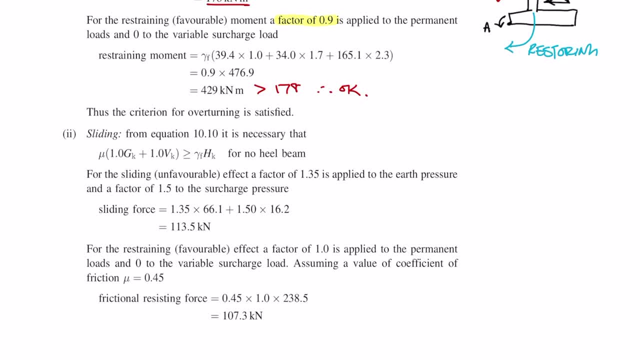 and this is just simply 1.35 times the dead and 1.5 times the live or the surcharge. Next, we want to calculate the frictional resisting force. by multiplying the co-efficient force by the coefficient of friction by the vertical forces, We can see that the resisting force is less than. 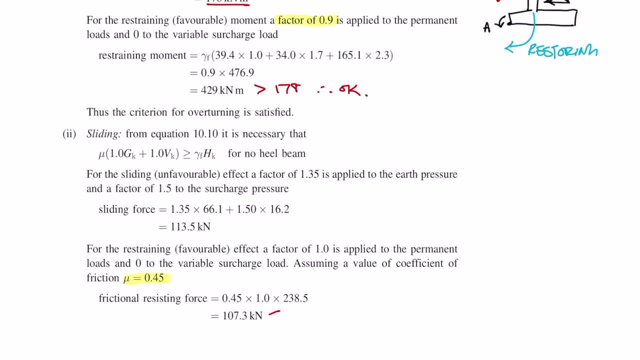 the applied sliding force. therefore, we need to use the heel beam and the passive pressure to increase the frictional resisting force. Using a heel beam is generally not very economical but for the sake of this design example, we'll go through it. The additional frictional force is very, very 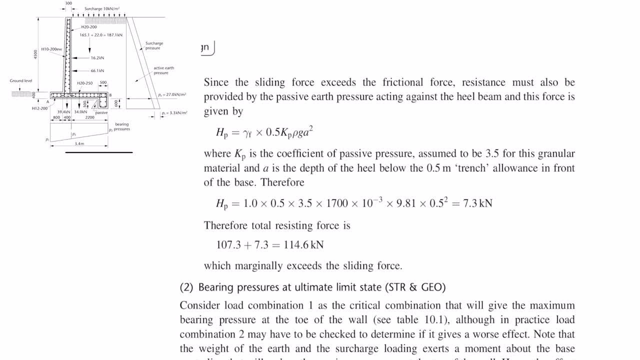 easy to calculate and all you really need is the coefficient of passive pressure, and in this case we're assuming it's 3.5 for granular material. and just like you worked out the horizontal force for the earth pressure, you basically do exactly the same calculation, except you're substituting in 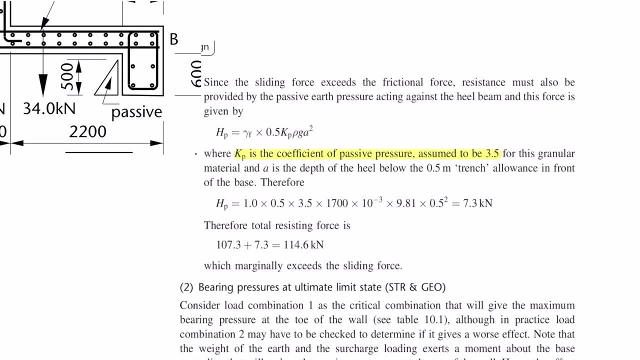 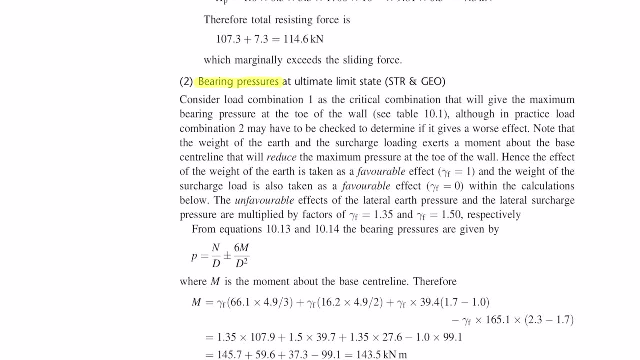 a different h value and the passive pressure coefficient. Add the two forces together and you will see that it marginally exceeds the sliding force. therefore the design passes. So now that we've done with the stability check, now we need to check what the bearing pressures are. So in a similar 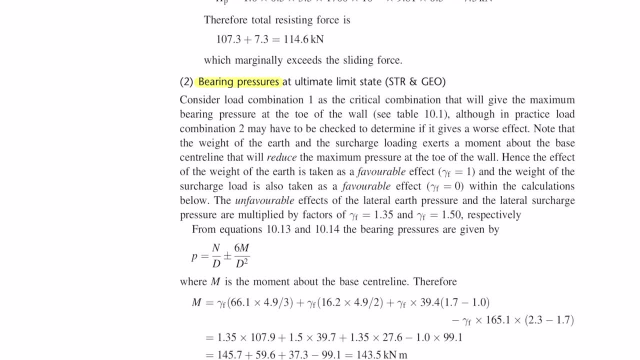 way in how we calculated the bending moments when we did the check for overturning. we need to find the moments about the base centerline, So the moments due to earth pressure and the surcharge is basically exactly the same as when we did it for the overturning check. What's slightly 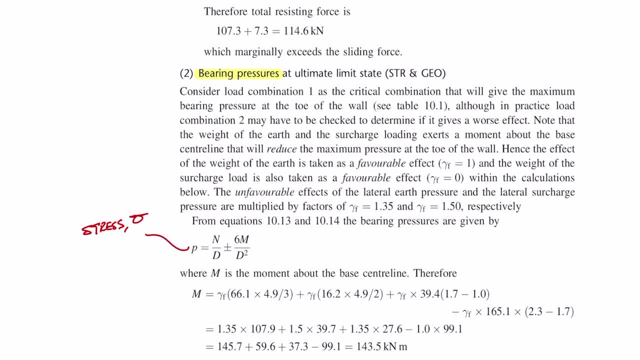 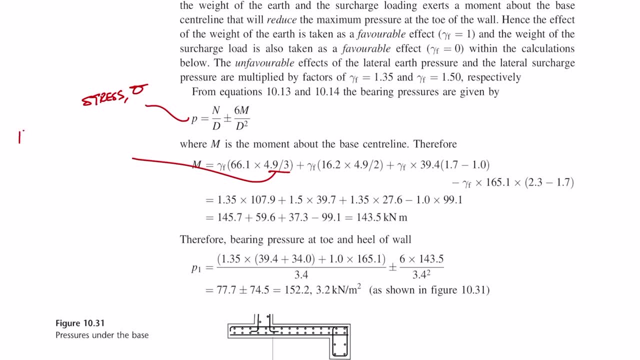 different is because of where we're taking moments. the weight of the stem is going to be additive to the earth pressure and the surcharge moments. So the lever arm between the center line of the base and the stem is 1.7 minus one. then we multiply it by. 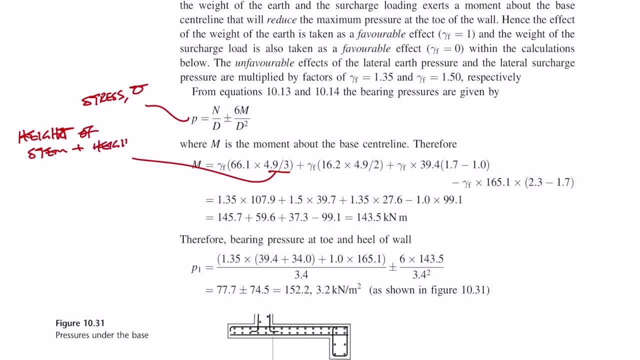 the vertical force or the vertical weight of the stem and we need to work out the bending moments due to the vertical weight of the soil. but this acts in the opposite direction, so we're giving it a negative sign. so the lever arm of the weight of the soil is basically the centre of mass. 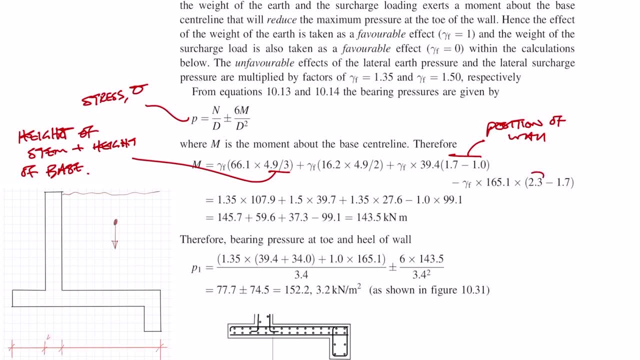 to the centre of the base And this should be 2.2, not 2.3 minus 1.4.. This means that the lever arm is the opposite of the base, so we're giving it a negative sign. So the lever arm of the weight of across the soil is basically to the centre of the base and it should be 2.2, not 2.3 minus one. 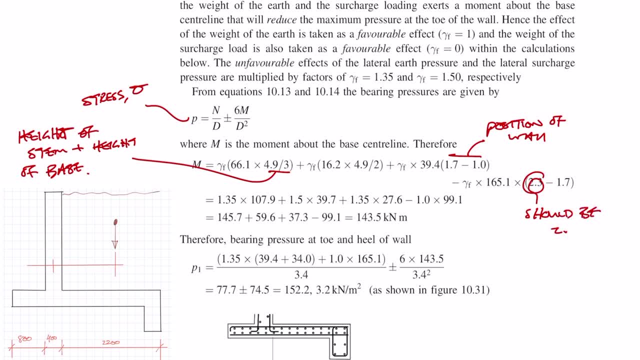 2.3 minus 1.7. the difference is pretty negligible. so we'll just continue with their numbers in the textbook. then we can apply all the correct safety factors. so 1.35 for dead, 1.5 for live, and we also apply one if it's a favorable effect. in this case, because we want the largest bending moment, we're 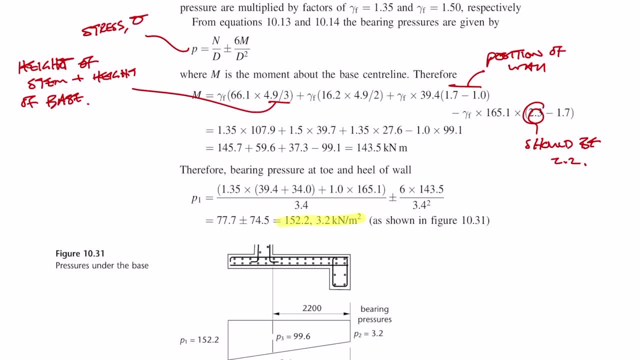 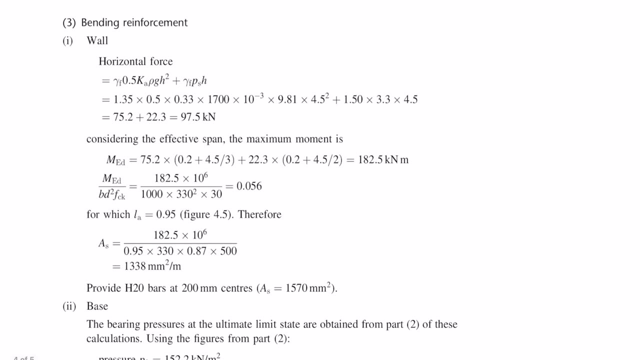 putting a factor of one against the negative bending moment. now that we've worked out the moment, we can plug in the actual force, the moments, into the stress equation to get two values of stress: 152.2 and 3.2. now we can move on to calculating the bending reinforcement in the wall. 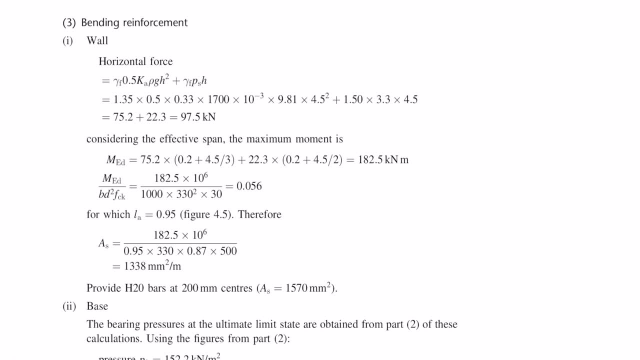 and the base. so the biggest bending moment in the wall is going to be at the base of the wall. so therefore, we're going to take moments about the base of the wall. so once you've worked out your bending moment, we also need to work out the effective depth before we can calculate the area. 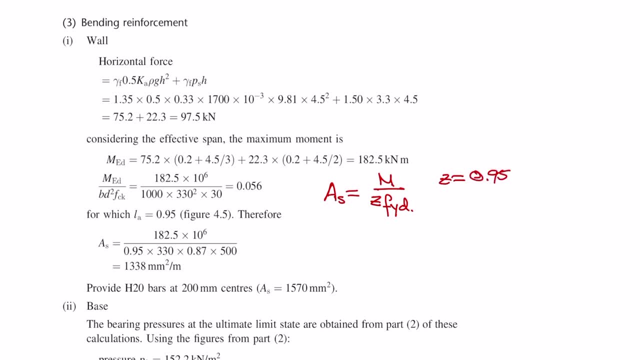 of steel required. the wall fitness at the wall is going to be at the base of the wall, so therefore we're going to take moments about. the base of the stem is a 400 mil in this example. they're assuming that the effective depth is 330. 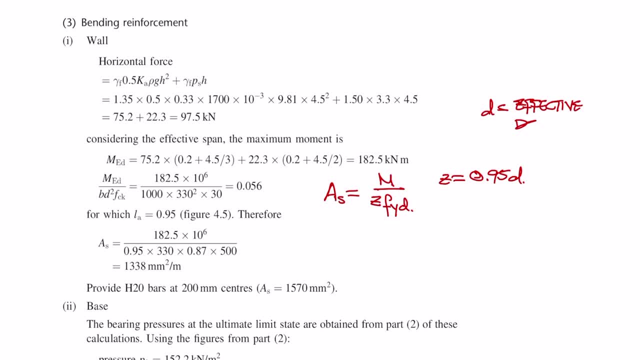 so therefore, the cover is going to be around 60 mil and the bars we're using is 20. if you want a more detailed video on how to calculate the cover, i suggest you go check out my reinforcement beam design video and, once you've got your effective depth, you should basically 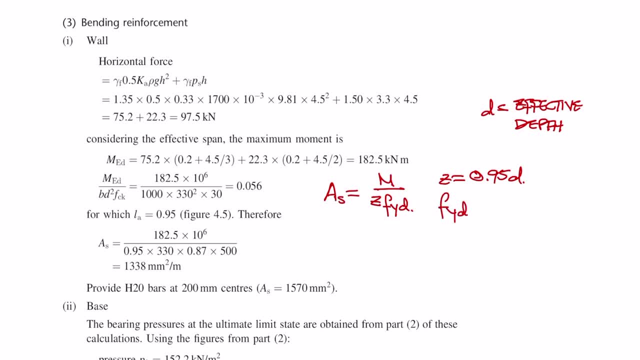 just plug in the numbers into this equation and then you get an area of steel required. then you want to specify a size of bar and the centers and this will give you your as provided. and as long as you're providing more than the required, then your design is more than adequate. 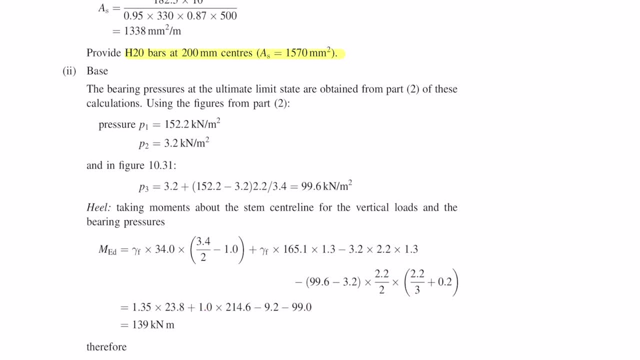 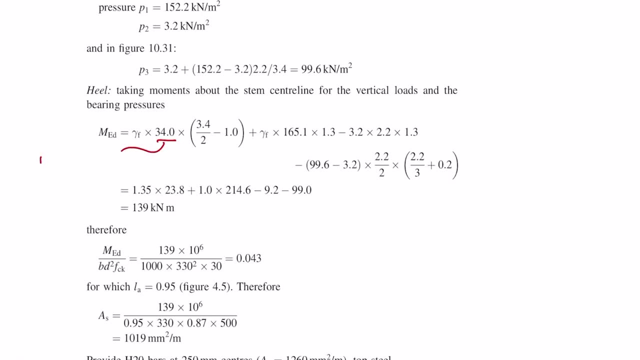 okay. so now we're moving on to calculating the base reinforcement, and we want to start by looking at the reinforcement at the heel, so we're going to be taking moments about the center line of the stem. so we're first calculating the self weight of the base multiplied by the lever arm, and that lever arm is the distance. 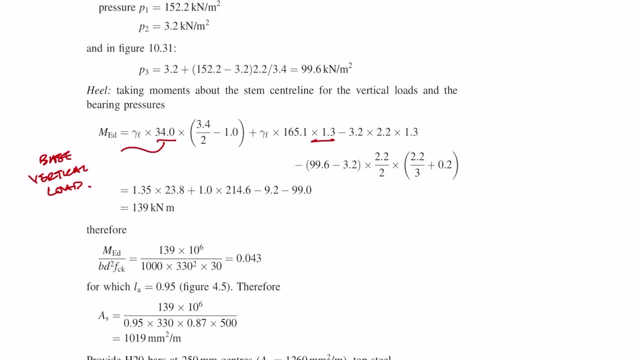 between the center of the base to the center line of the stem. then we want to do a similar calculation with the vertical load of the earth, and the lever arm in this instance is 1.3 meters. this next part is quite confusing, so i'm going to overlay a diagram of me doing this, and it's 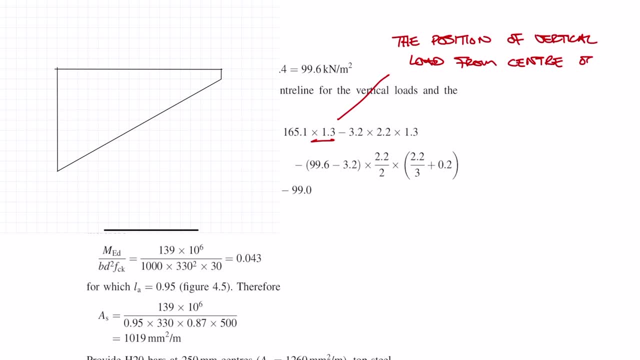 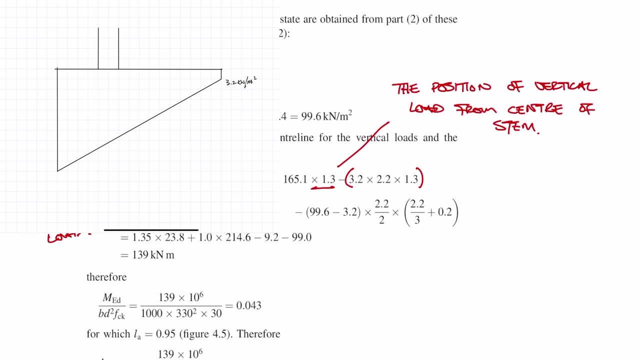 essentially working out areas and then multiplying by the lever arm again. but it's working out of these areas, which is confusing by just looking at the numbers. so what i'm doing is drawing a stress diagram, but to slightly more of a scale, and then we're working out the stress at the face. 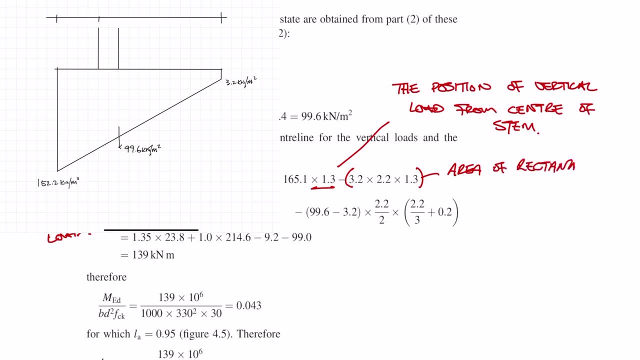 of the wall. so first of all, i'm going to work out the bending moment. due to the stress of the rectangle in red, and because it's a rectangle, the resultant force acts in the middle of the rectangle. so we know that the resultant force is 2.2 divided by 2, and to get to the center line of 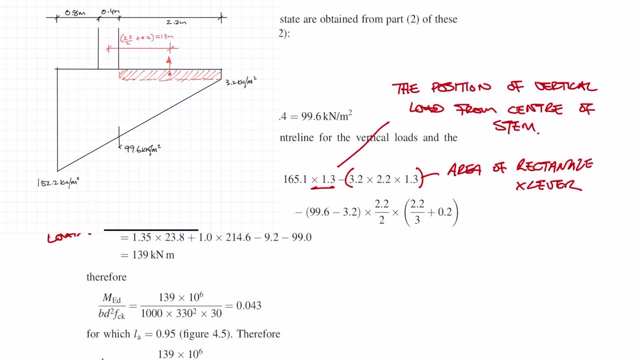 the stem, we need to add 200 mil. so therefore the lever arm is going to be the center line of the rectangle and the lever arm is 2.2 divided by 2 plus 0.2, which gives us 1.3. so now we need to. 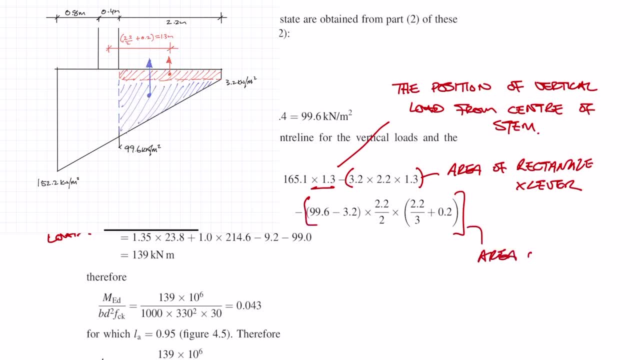 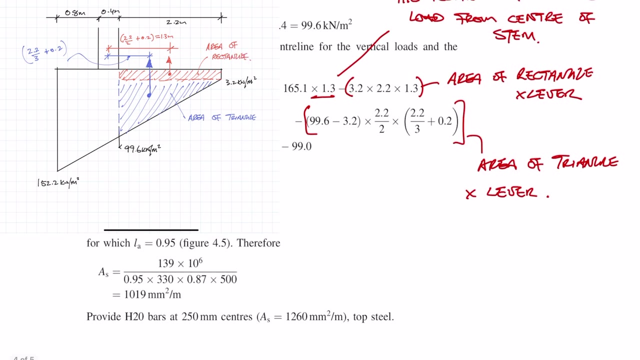 calculate the moment. due to the remaining stress, which happens to be this blue triangle, and because it's a triangle, the resultant force acts a third of the way from the wall. therefore, the lever arm is 2.2 divided by 3 plus 0.2. so in both instances we're multiplying the area of the triangle or the.